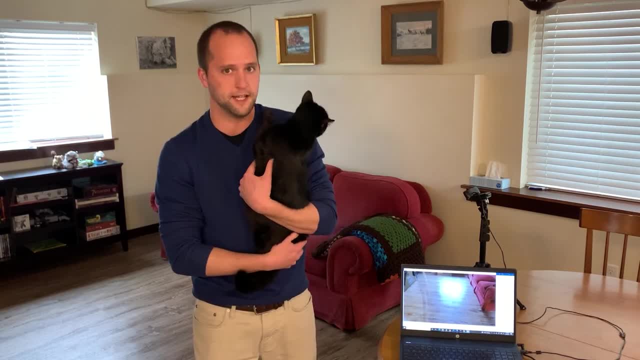 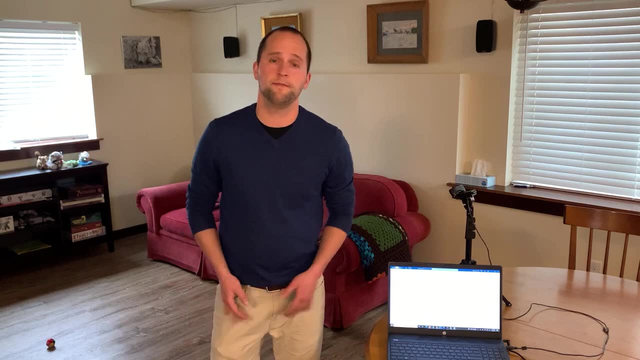 detection model on frameworks like TensorFlow. as I show in my other videos, The first step for creating any machine learning model is to build a data set For object detection models. this means capturing and labeling hundreds to thousands of images of the objects you'd like to detect Now. 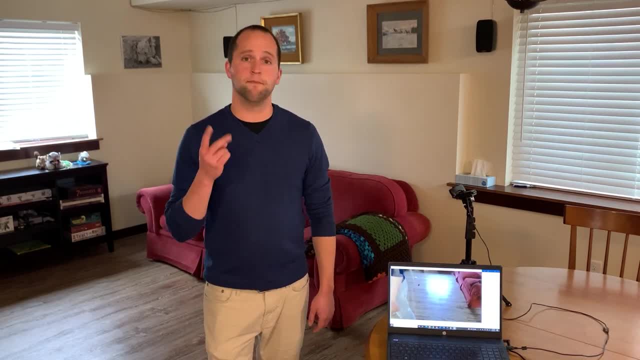 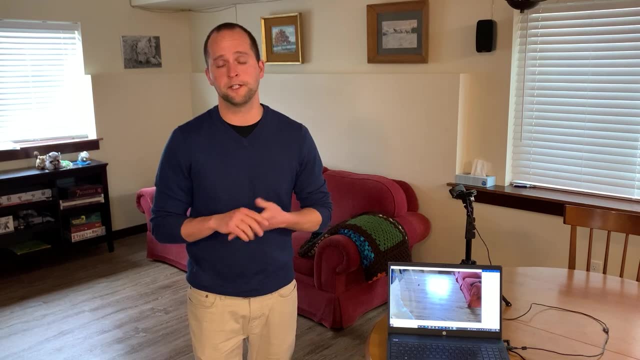 it turns out that building a data set is actually the hardest and most important part of the process for training a model. There's tons of details that should be considered as you're going around gathering pictures, but for this video I'll just show the basic process for taking pictures of 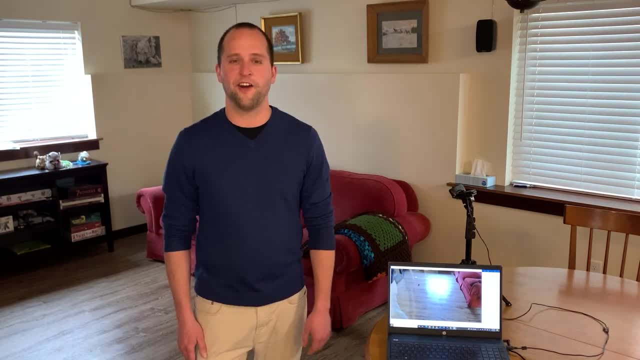 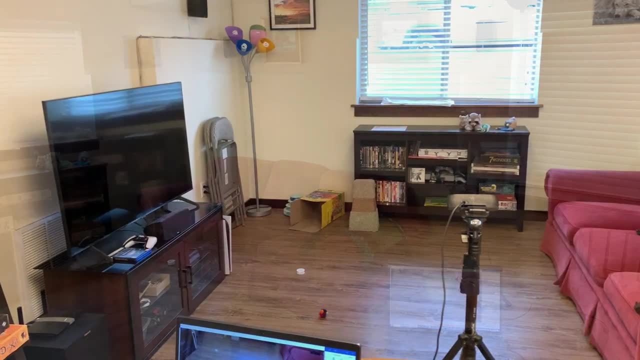 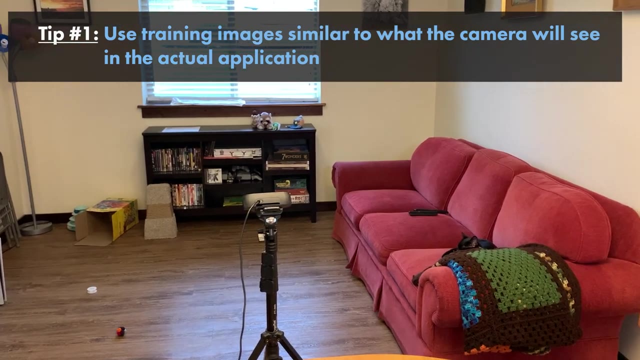 your objects and labeling them using label image. All right, come on, Cleo, let's get started. Before you start gathering images, it's important to think about your object detectors application. You want to think about the environment. it will run in the perspective and distance it will see. 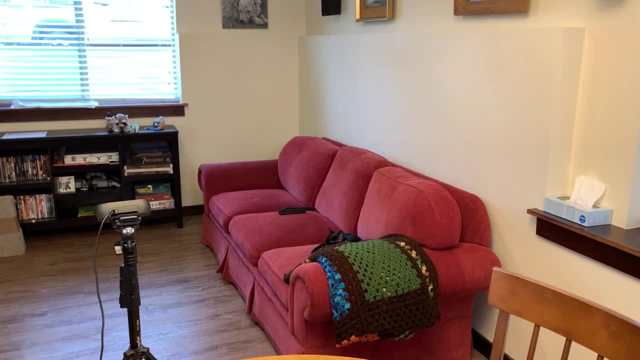 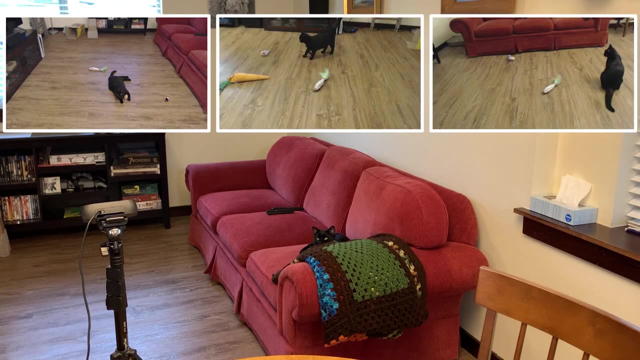 the objects from, and even what type of camera it will use. The pictures you take should be similar to what the object detection model will actually see when it's deployed in your application. If it will be used in a variety of locations and conditions, you'll need to get 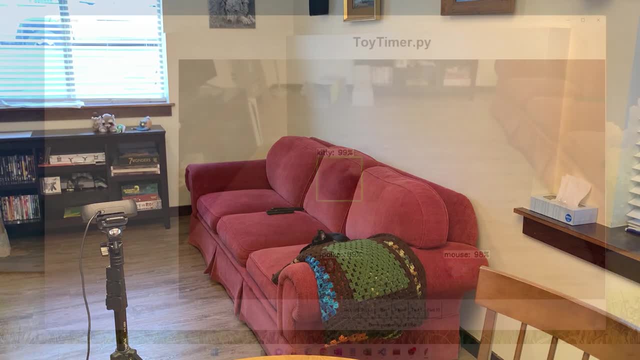 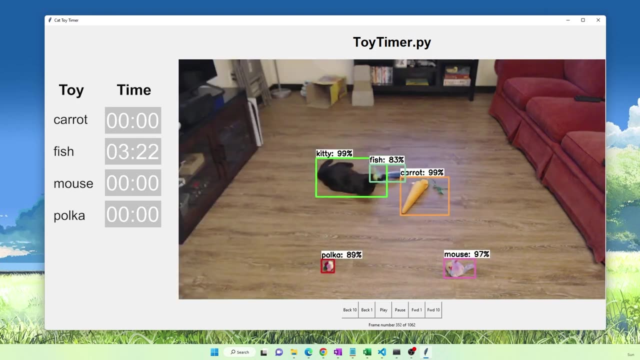 training images that represent those locations and conditions For this video. the application I'm working on is a cat toy timer. I just got Cleo a bunch of new toys and I want to set up a camera to watch Cleo as she plays with them. It'll keep track of how much time she spends playing. 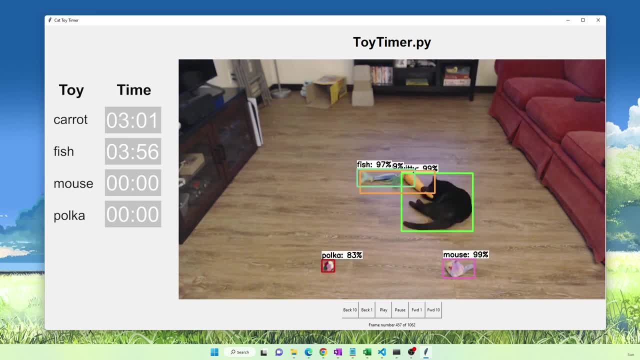 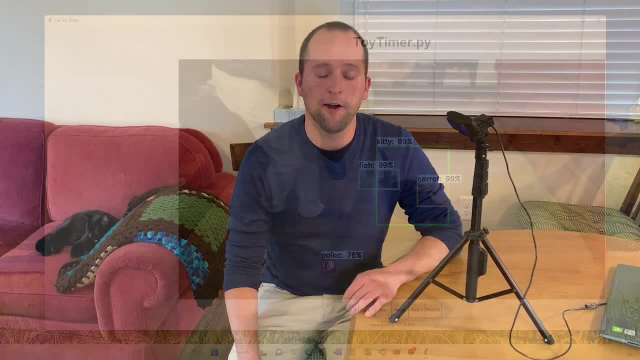 with each toy. That way I'll know which one's her favorite so I can buy her more. I'll work through the data gathering process to see if I can get a better idea of what the object detection model will do. The first step is to start with the camera. Set up the camera so it's pointing at the area where you. 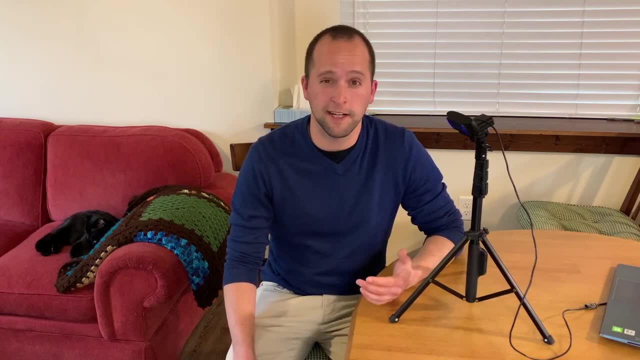 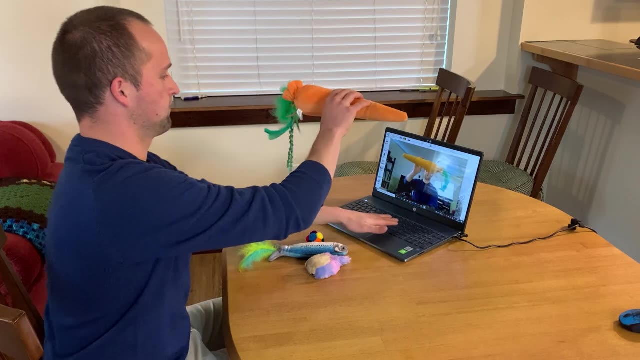 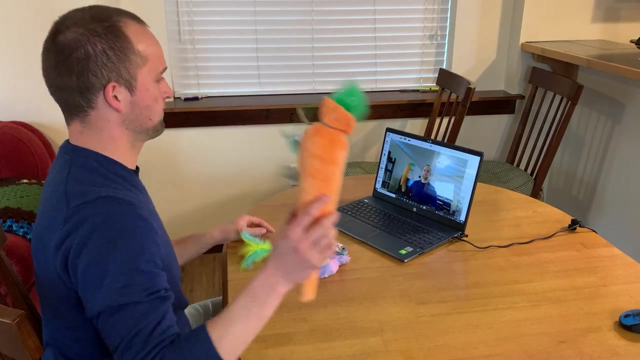 want to detect your objects. This step can vary in complexity depending on the scope of your application. If you just want to detect objects in front of the camera, you can make a simple setup where you set or hold objects in front of the camera at various angles and distances You can hold. 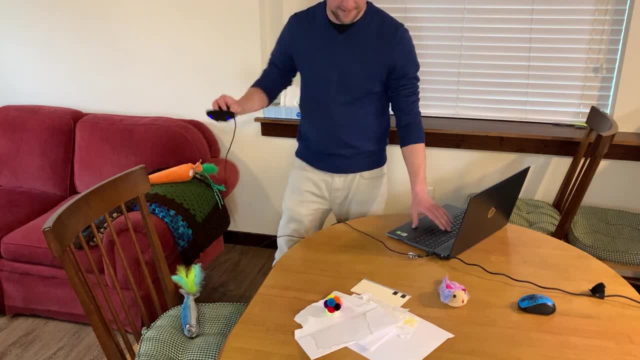 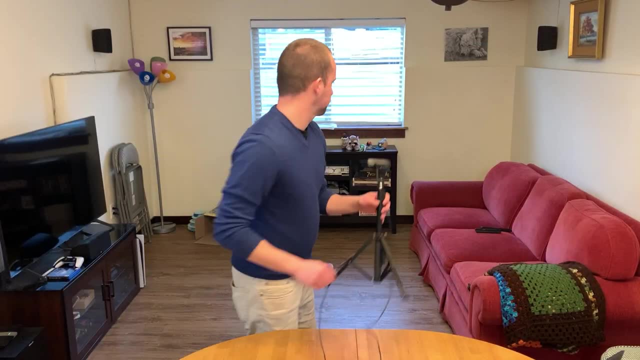 You can hold the camera and walk around taking pictures of the objects you want to detect, Or if your application is going to see the objects from many different perspectives and backgrounds, then you'll need to set up the camera in a variety of ways to capture multiple. 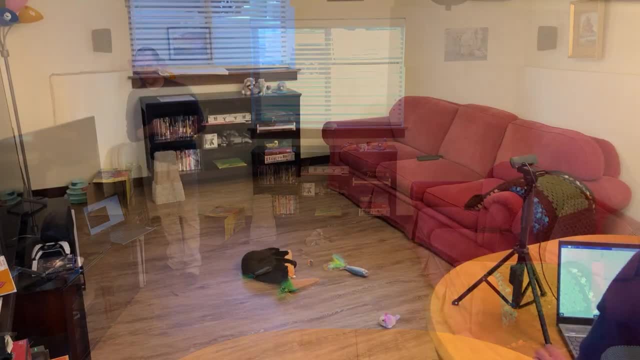 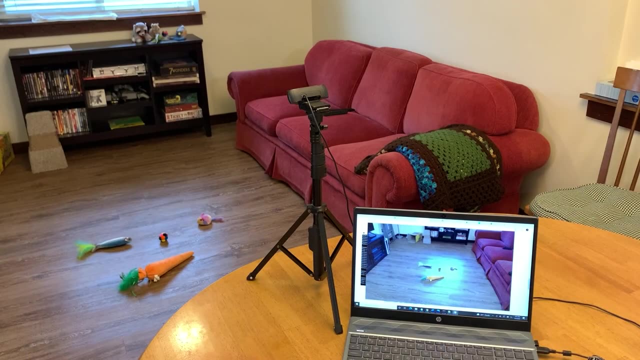 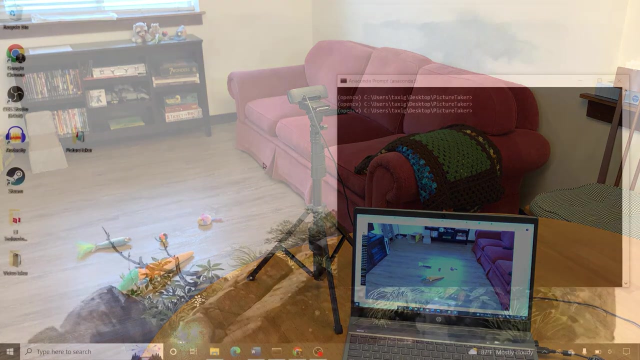 views of your objects For my application, I'll set my camera up to point at the floor where Cleo usually plays with her toys. Okay, now that your camera's set up, let's take some pictures of the objects. You can use any picture-taking software that's installed on your computer. 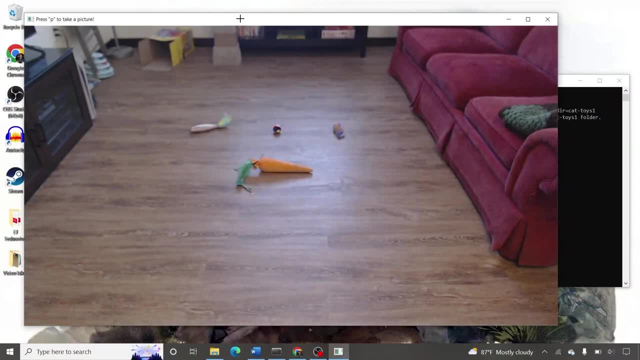 If you've got OpenCV set up on your computer, you can use a simple Python script I wrote called PictureTaker. It will open the camera and take a picture anytime you press P on the keyboard. Each picture will be saved into a specified folder. 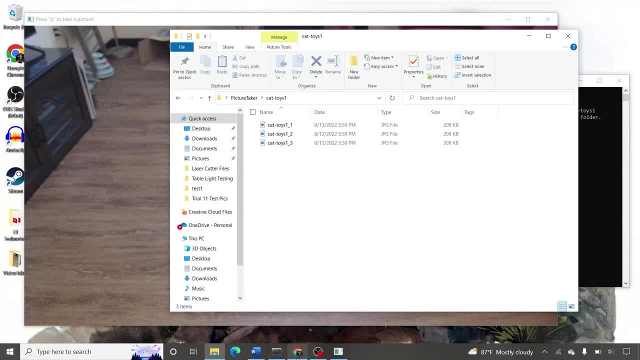 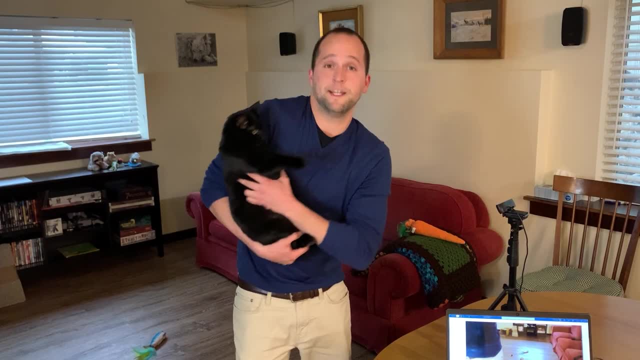 Instructions on how to install and use PictureTaker are available on my GitHub, See the link in the video description below. So the goal of taking pictures is to provide enough statistical data to the machine learning model for it to learn what your objects look like. 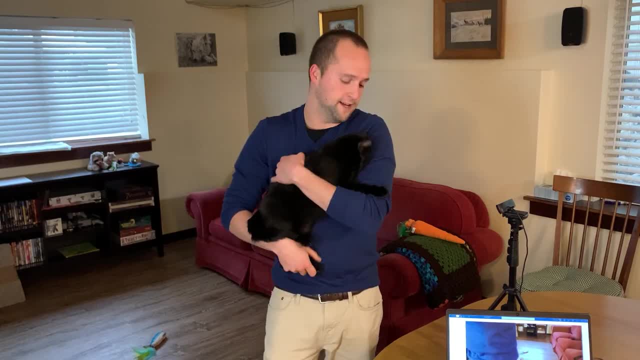 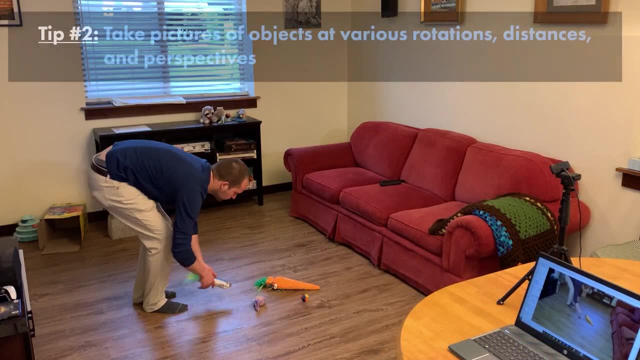 For an initial model, you want to have at least 200 pictures in your data set. You should have at least 50 examples of each object, Set objects in the camera's field of view and take pictures of them at different rotations, distances and angles. 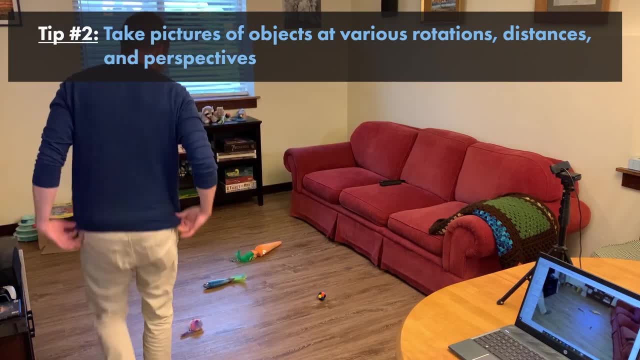 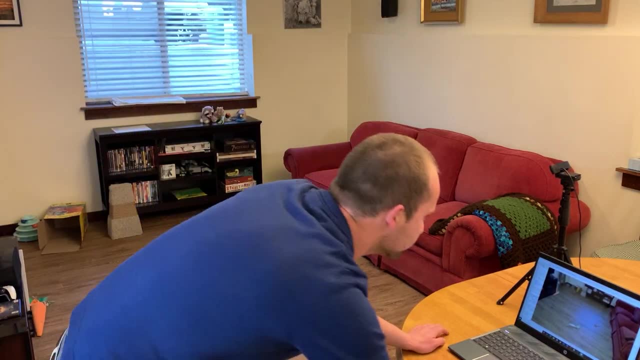 In my case, I'm going to set the pet toys on the floor, take a picture, reposition the toys and repeat. I'll change the camera's location, height and angle a few times to get a different perspective of the scene. 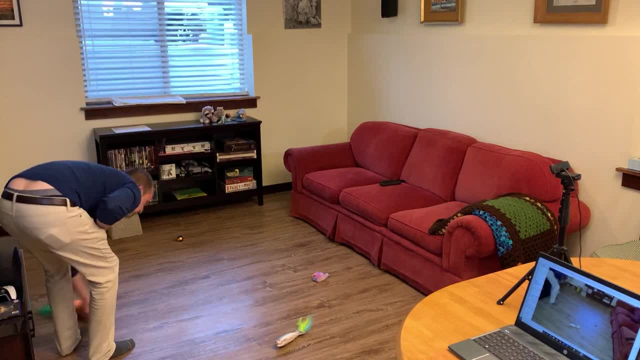 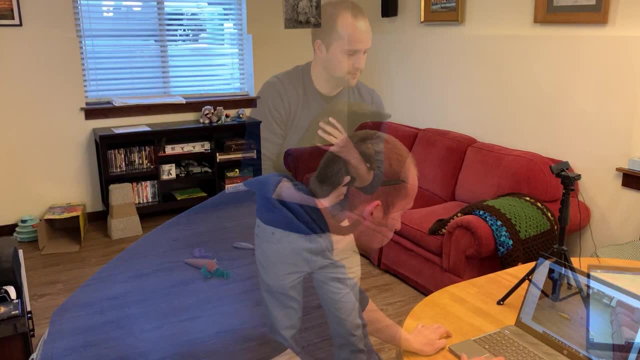 If you know you'll be detecting objects in scenes with busy backgrounds. you can also include other objects in the pictures or use various backgrounds to improve robustness. And of course I need pictures of Cleo too. I'll let her play with the toys and take pictures while she's playing. 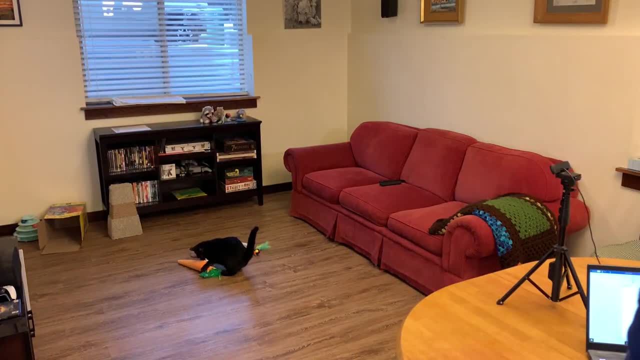 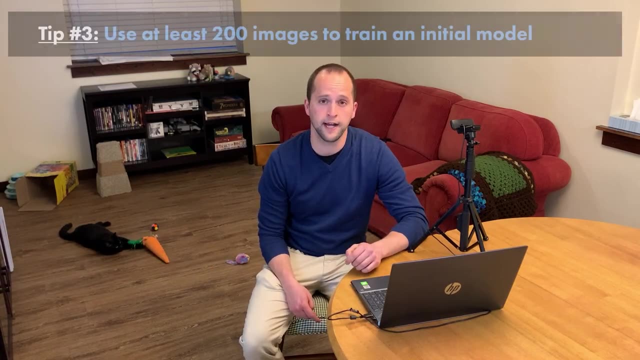 Go get them. Cleo: Once you've taken a picture of Cleo, you'll want to take a picture of her while she's playing. If you've taken at least 200 pictures, you should have enough to train an initial model. 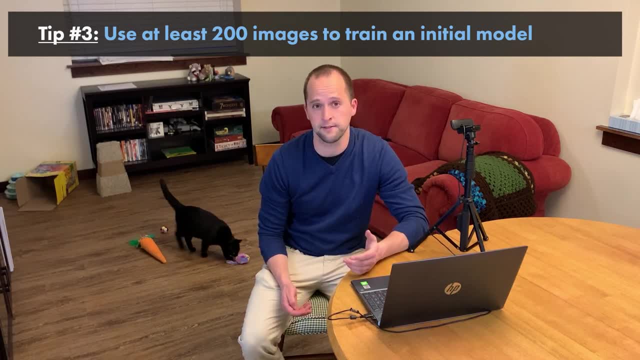 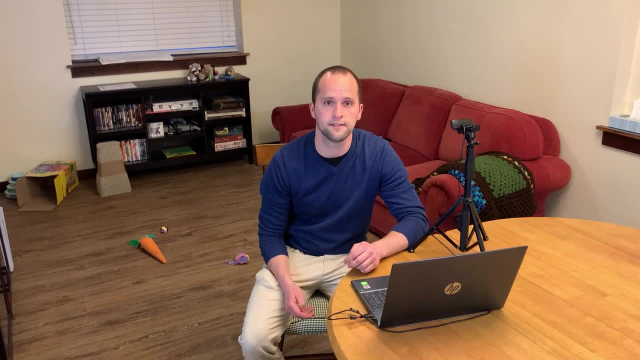 If you really want to go crazy, you can take 500 or even 1,000 pictures. Production quality models actually will end up using 10,000 to 100,000 or even a million images, So the more pictures that you take, the more accurate your model is likely to be. 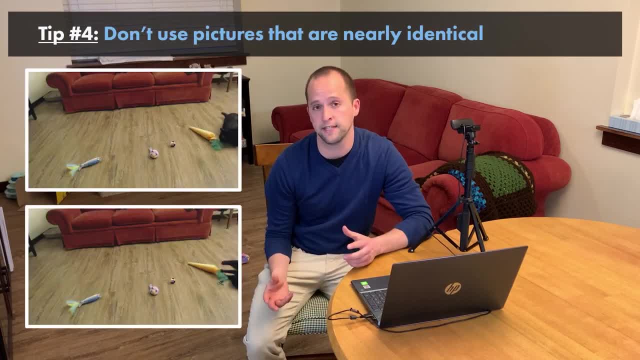 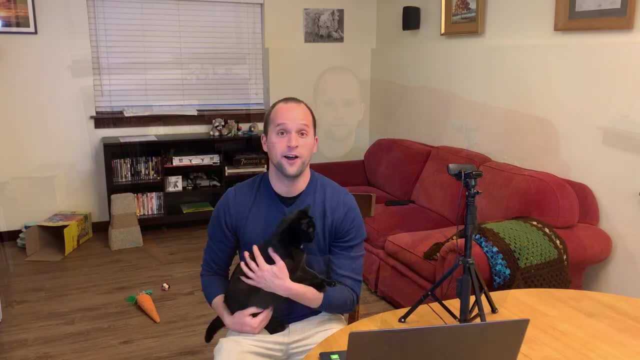 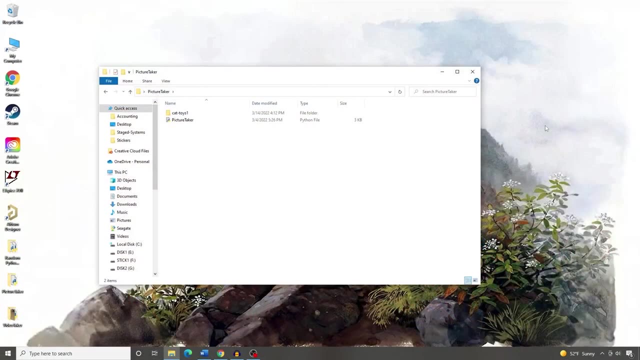 But make sure that there's enough visual difference between each picture you take, or else these additional pictures that all look the same won't provide much value to the model. Okay, we're finally done taking pictures. Now it's time for the fun part: labeling them. 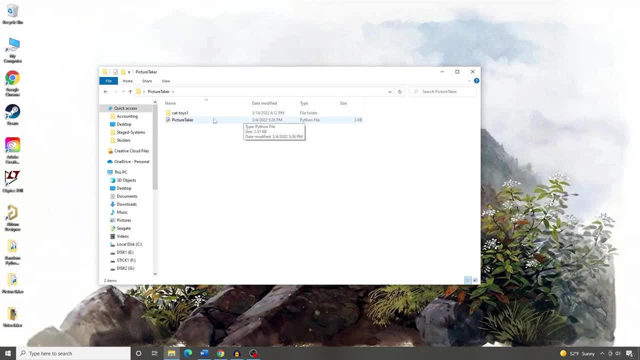 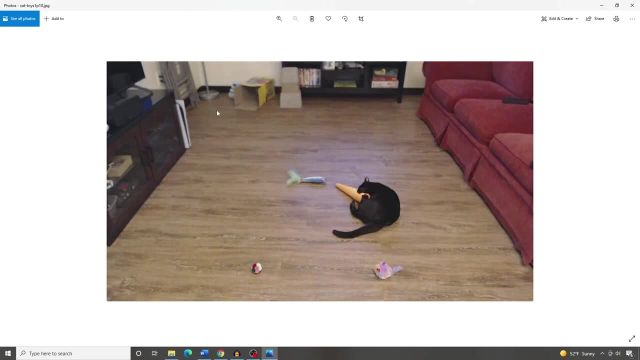 Let's switch over to the computer, where your images are stored. At this point you should have a folder full of pictures of your objects. Now we need to label the class and location of each object in every image. The training algorithm will use this label data to teach the model what your objects. 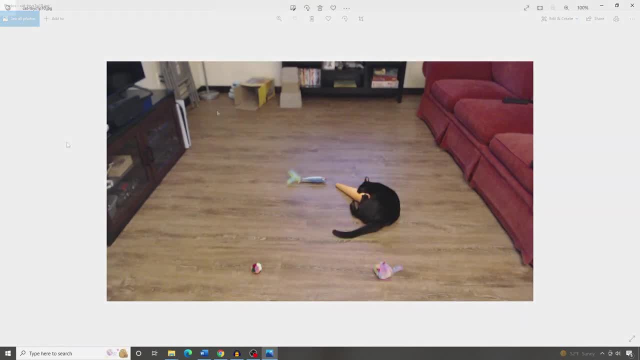 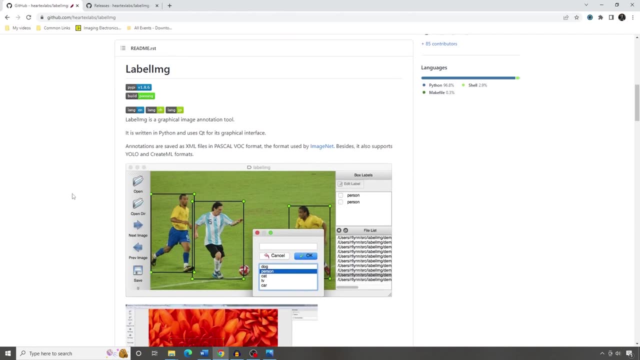 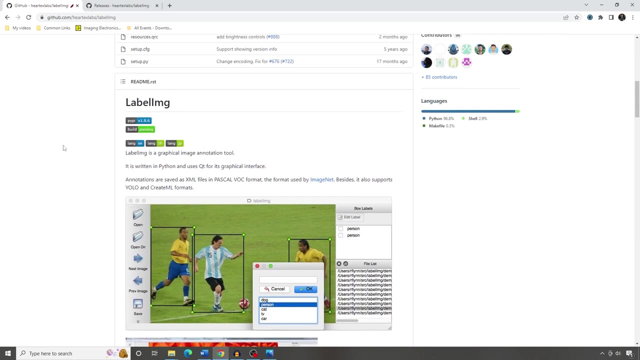 look like and how to locate them in future images. Okay, To annotate the images, we'll use an open-source labeling tool called Label Image. Label Image has a simple and effective interface for drawing bounding boxes around objects and indicating their class. Label Image is pretty easy to install. 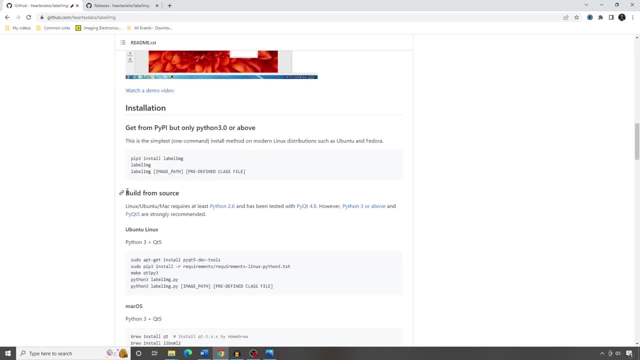 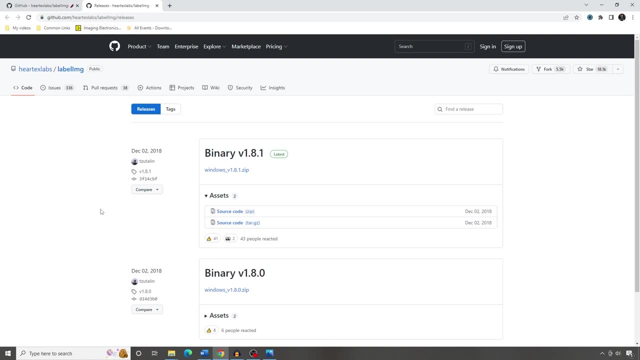 If you're on Linux or Mac OS, follow the instructions on the GitHub page For Windows. Label Image is available as a standalone executable. Install it by going to the releases page linked in the video description below and downloading the Windows file for the latest version. 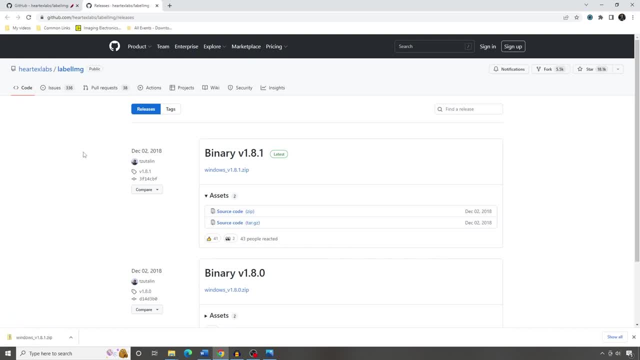 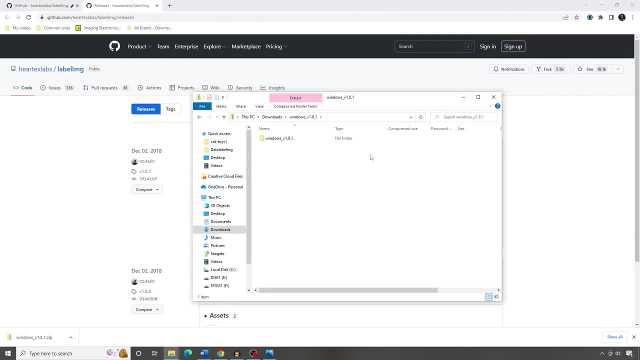 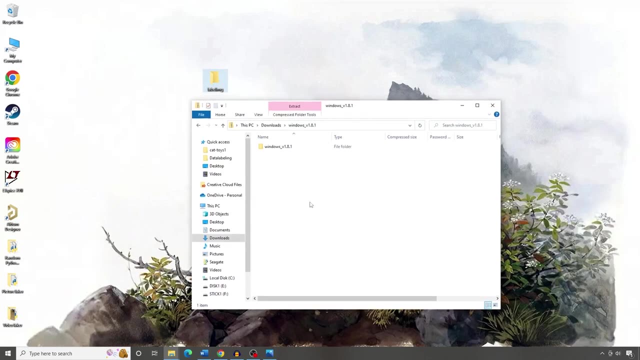 Now we're ready to go. Next, go to your Downloads folder. Label Image comes in a zip file that can be extracted to wherever you'd like on your computer. I'll create a folder called Label Image on my desktop and then copy the folder inside. 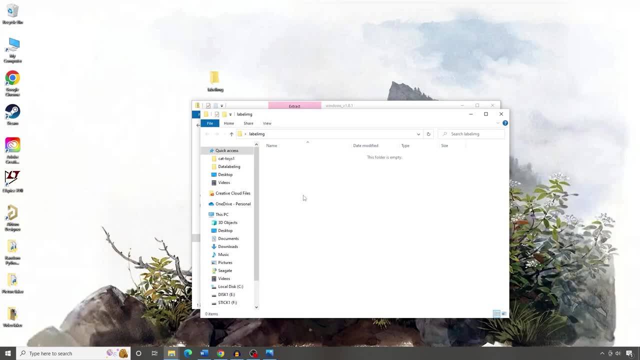 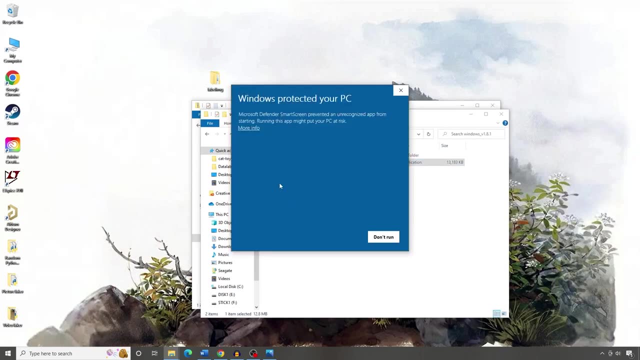 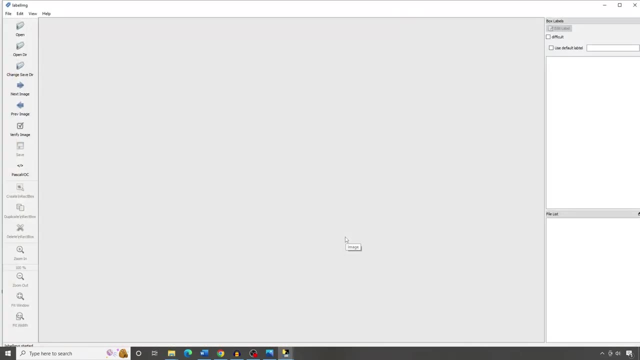 the zip folder into the Label Image folder, Then go into the new folder and double-click the Label Image executable. Windows might try and stop it from running. If it does, just click More Info and then Run Anyway, All right, This is Label Image. 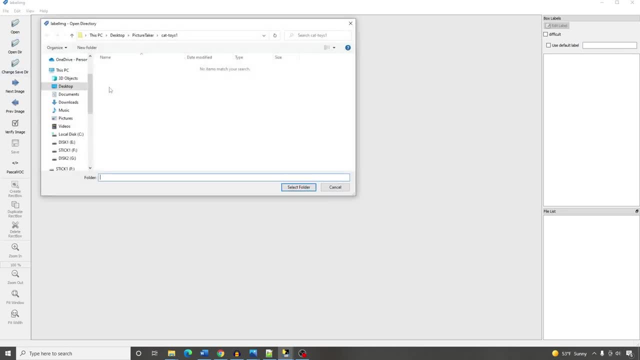 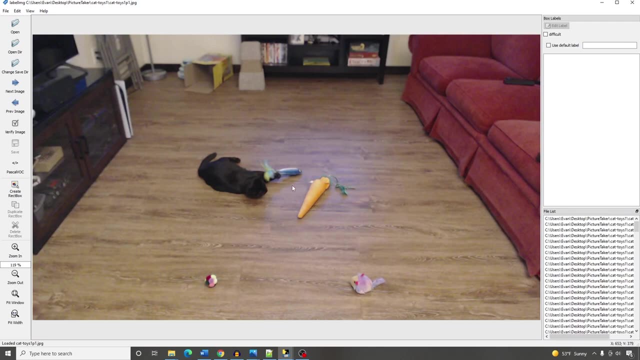 First open your folder of images by clicking the Open Directory icon and navigating to the folder where your images are stored. Click the Select Folder button and the first image in the folder will appear. Time to label some objects. To start drawing a box, click the Create Rect Box button and click to draw a box around. 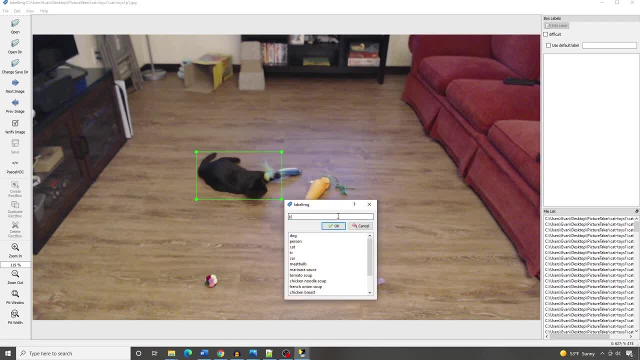 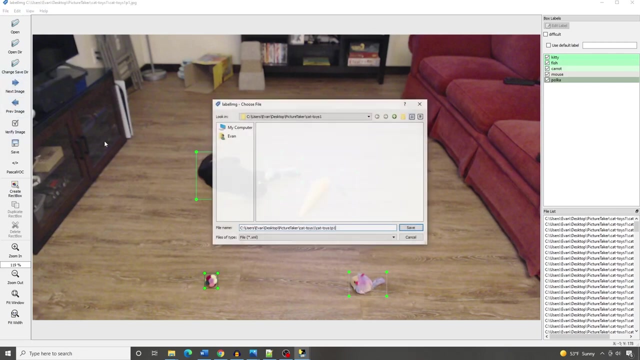 the first object in your image. Type in the name of the class and click OK to complete the label. Repeat the same process for each object in your image. I'll give some more tips on good labeling practices later in this video. Once you've labeled all the objects, click the Save icon and just save it as the default. 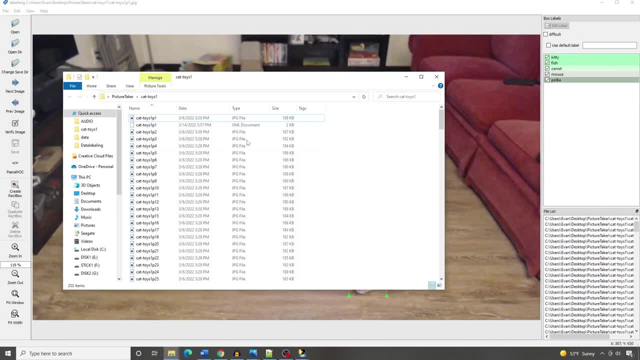 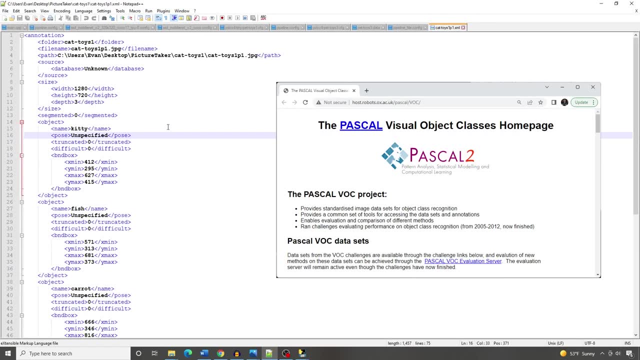 file name. This creates an XML file inside the folder. This creates an XML file within the folder. file contains annotation data for the image. the data is formatted in the pascal voc annotation format, which is a standard way of storing bounding box coordinates, classes and other information. 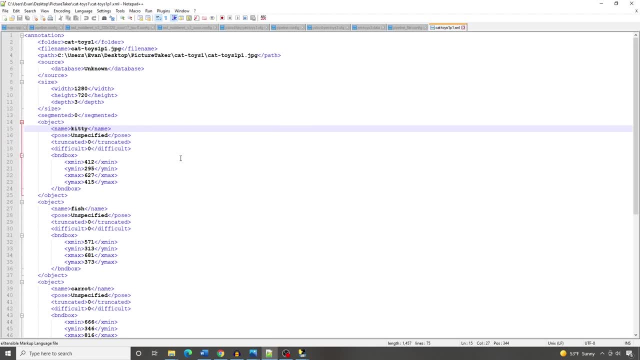 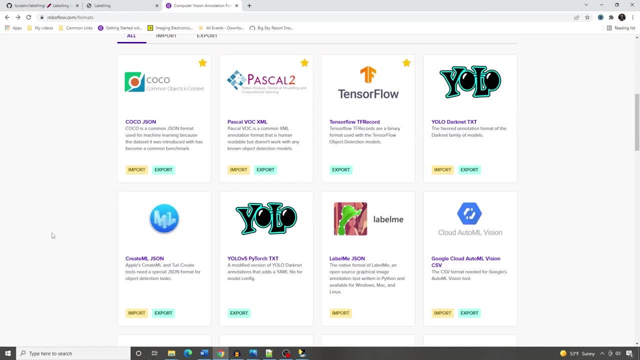 about objects in an image. this format is commonly used with the tensorflow object detection api to train models. if you're using a different framework, the data can be converted to other formats using conversion tool like roboflow. go check it out if you're interested. okay, back to labeling. 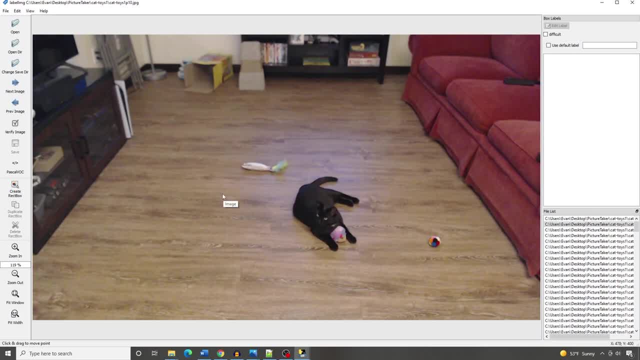 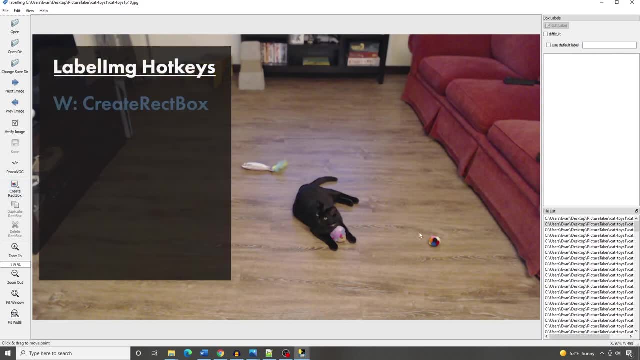 click the next image button to move on to the next image. now let's learn some hotkeys to help speed up the process. instead of clicking the create erectbox button, you can just click press w on the keyboard to start a new label box. instead of clicking on the save icon, you can just press control s to start a new label box. 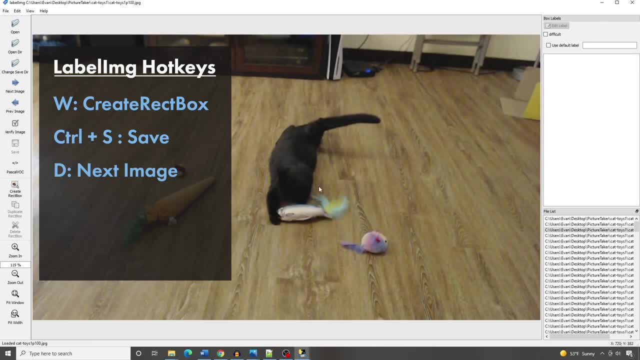 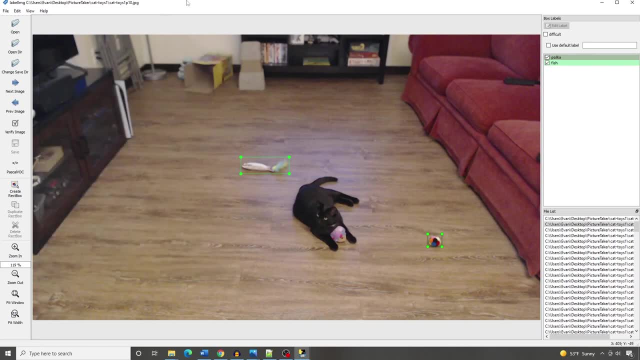 save a file, Press D to move on to the next image or A to go to the previous image. Another way to speed things up is to predefine the label map. Go to the folder where label image is installed and go into the data folder and open the. 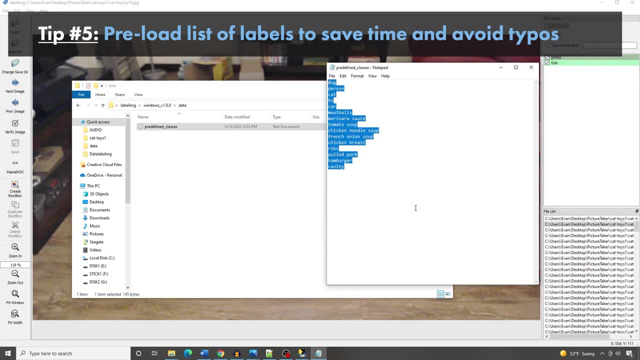 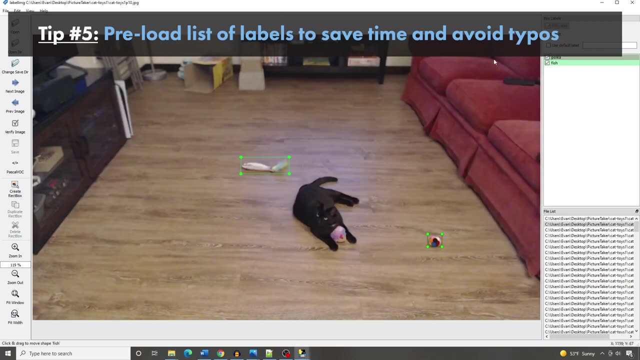 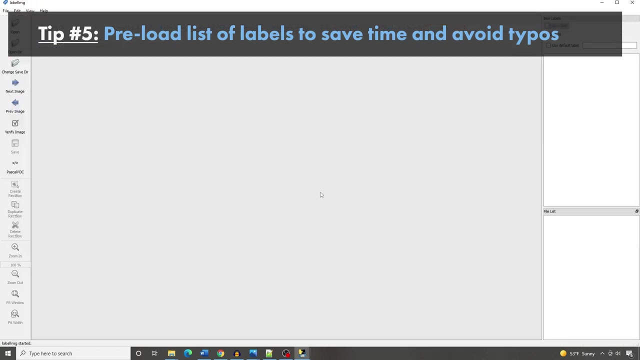 predefined classes file. Delete the existing classes and type in your own classes. In my case the classes are kitty, carrot, mouse, fish and polka. Then save and exit the text file. Now go ahead and close and reopen label image. Go back to. 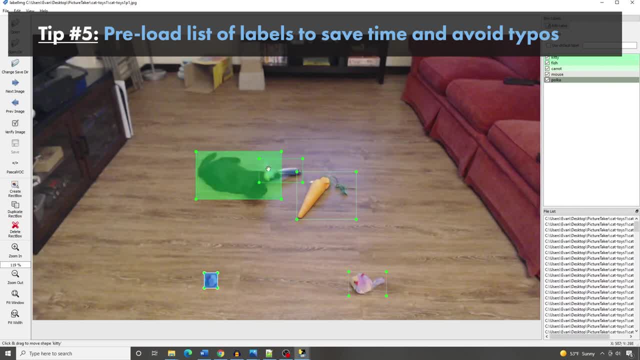 the directory where your images are stored. Now, when you draw a label box, the suggested classes will be the ones you put in the text file. This makes it so you don't have to type out the whole class every time. It also helps to prevent you from misspelling classes or using inconsistent class. 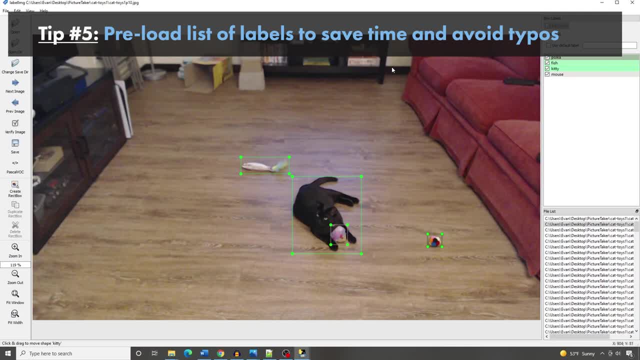 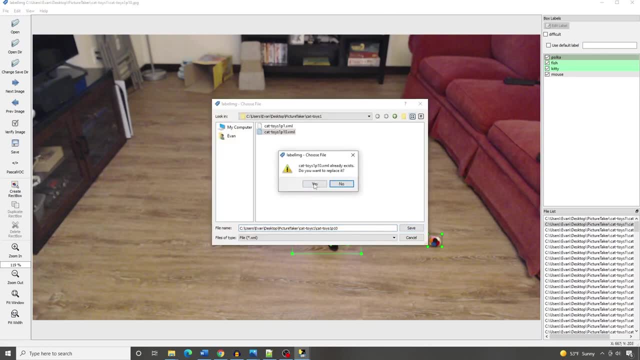 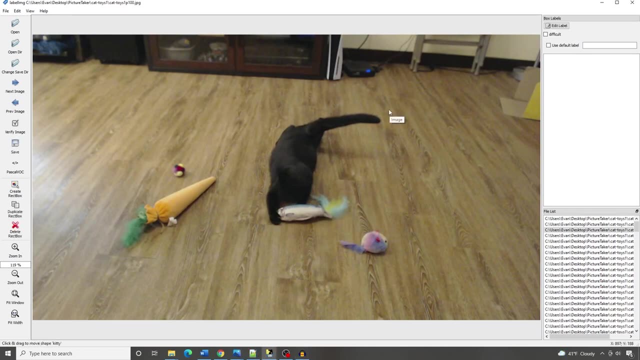 names, which can cause errors or performance issues during training. Make sure to save before going on to the next image. if you've made any changes, All right, let's go through a few more images and I'll give some labeling tips that will help your model achieve better performance. Object detection works best. 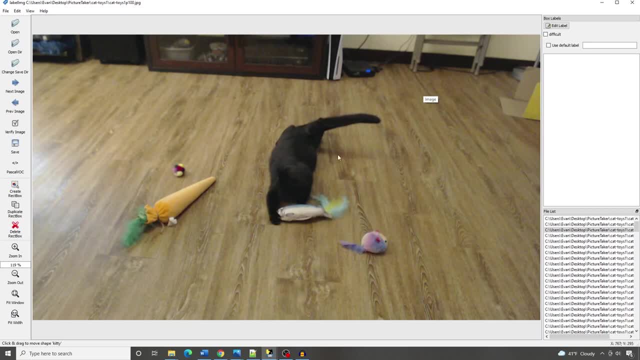 with a lot of different types of labels. For example, if you want to use a label box, you'll want to use a label that has clear and well-defined boundaries, like a cat or a vehicle. As such, make sure to include the full object inside the 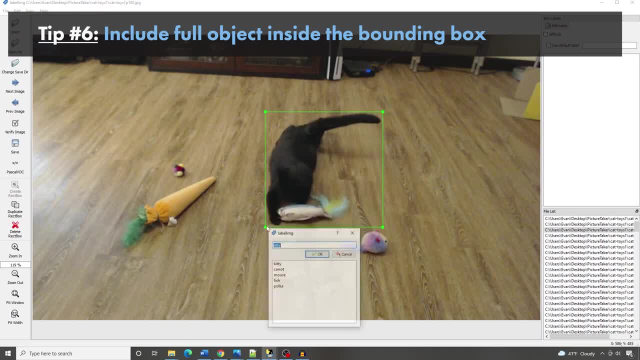 bounding box. It doesn't have to be perfect, but err on the side of making the box too big to make sure that the whole object fits inside the box. It's okay if there's a few pixels between the box and the edge of the actual object. You can. 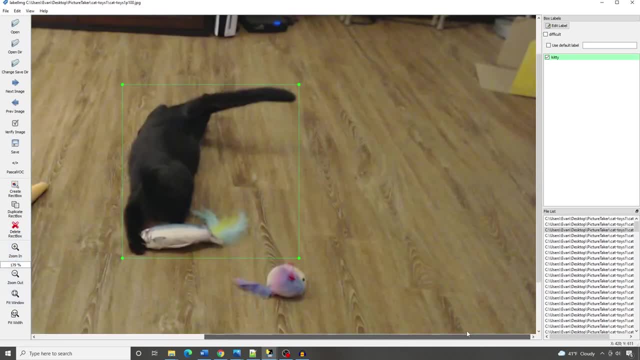 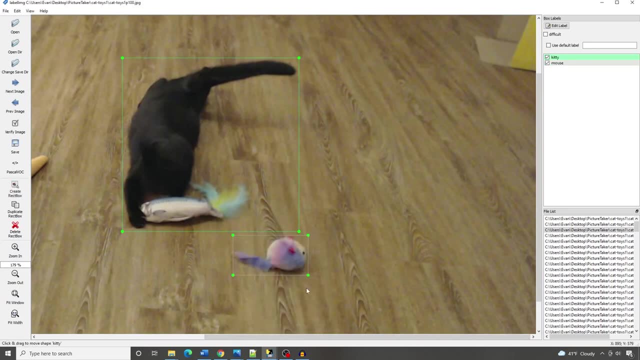 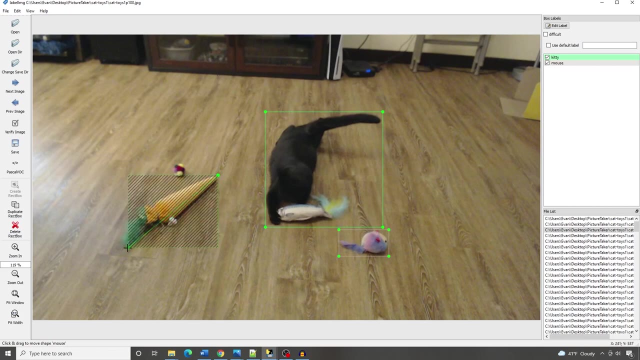 also use the zoom tool to draw a more precise bounding box around the object. So if the object is long and diagonally oriented in the image, that means you'll get a lot of background when you draw a box around it. but that's okay, Just make. 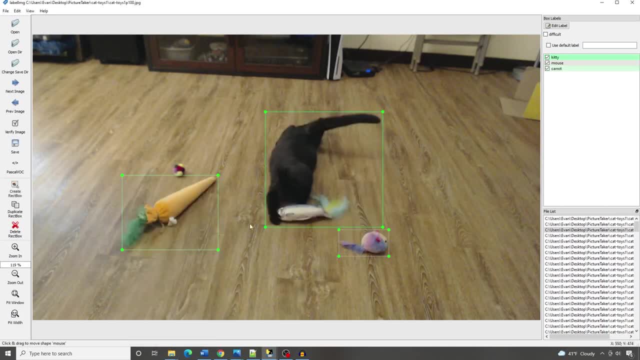 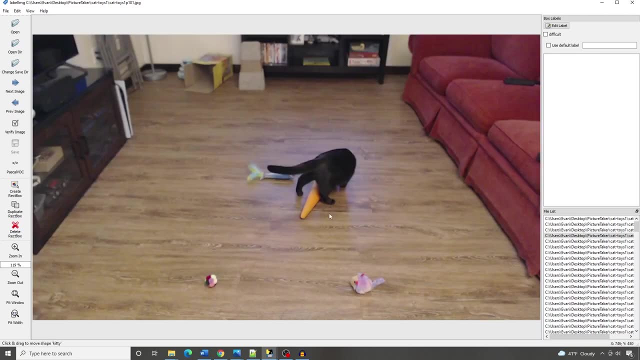 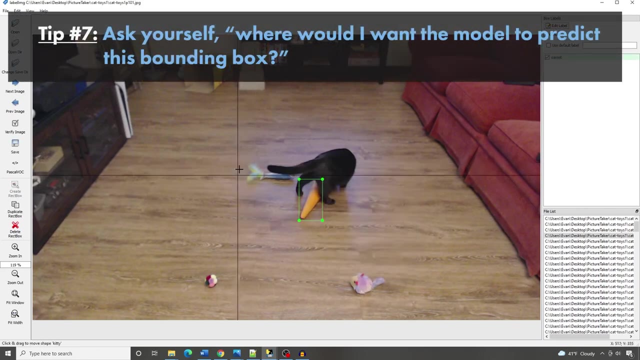 sure to have multiple examples of this object in multiple orientations in various images. If an object is partially obscured, like this carrot, is just draw a box around the part that's visible. A good way to think of how to draw bounding boxes for obscured objects is: where would I want the model to predict this? 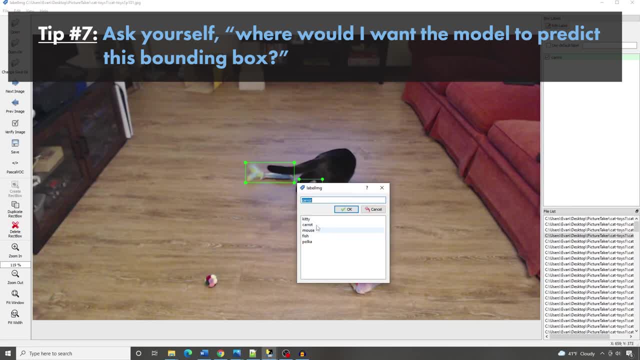 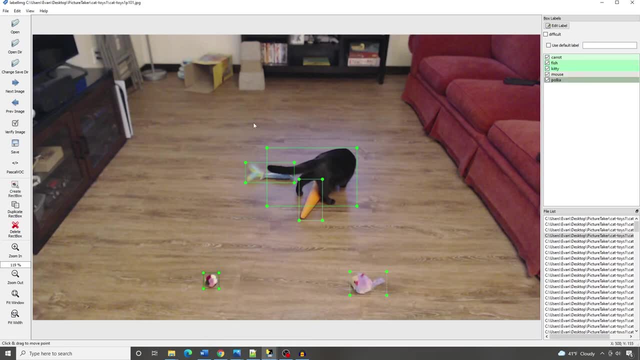 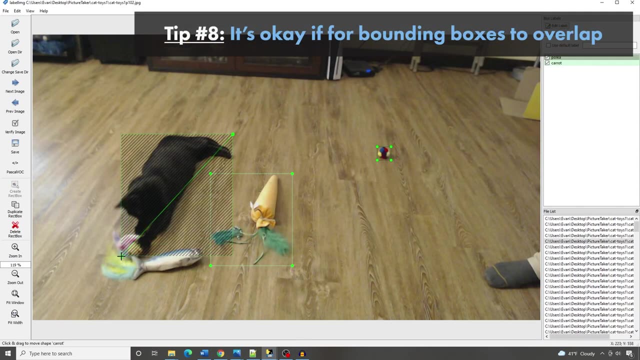 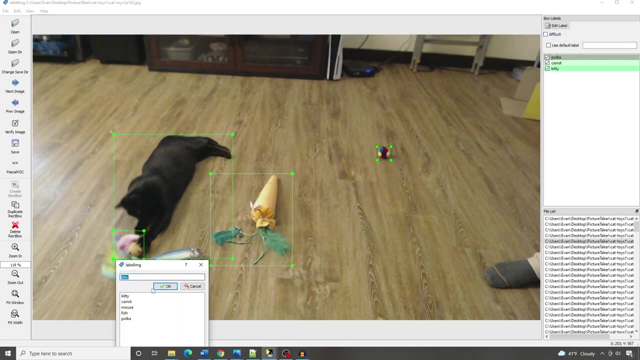 object's location. Wherever you want the model to predict the location, that's where you should draw the bounding box. It's also okay for bounding boxes to overlap, so don't worry if the bounding boxes intersect each other. However, avoid using images that. 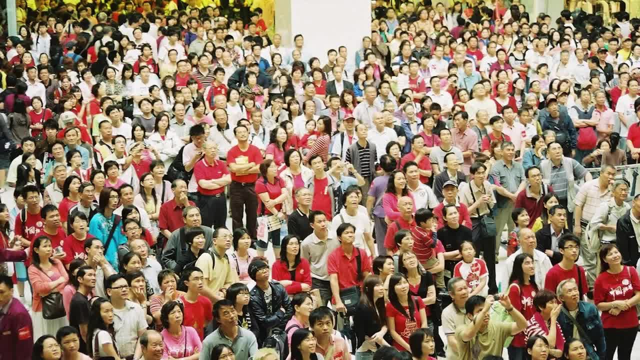 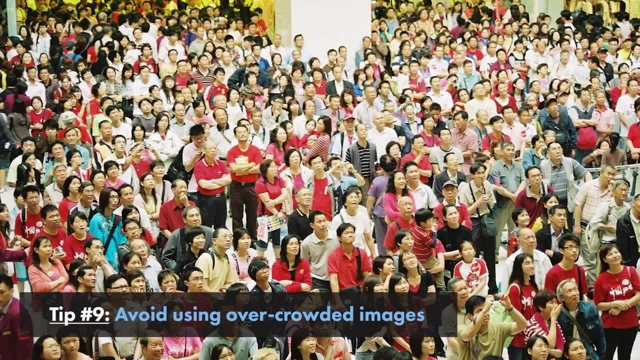 are too cluttered with objects. Here's an example picture of a crowd of people. Say you want to train your model to detect and count each person. How would you label this image? It's hard to define where the edge of each person is. As such, 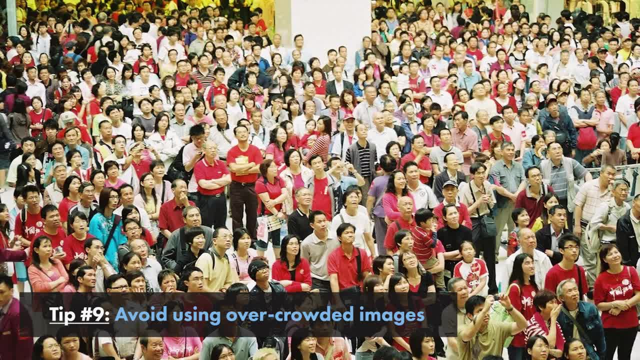 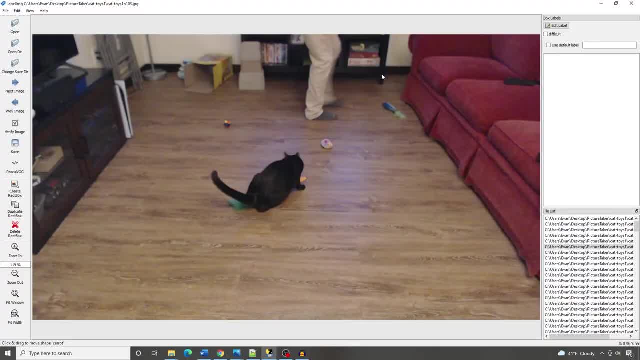 your model will have a hard time predicting bounding boxes. It's best to use images where there are clear boundaries around each object. In some images it's hard to know what the bounding box for an object should look like or whether it should even be labeled. For example, I can barely see 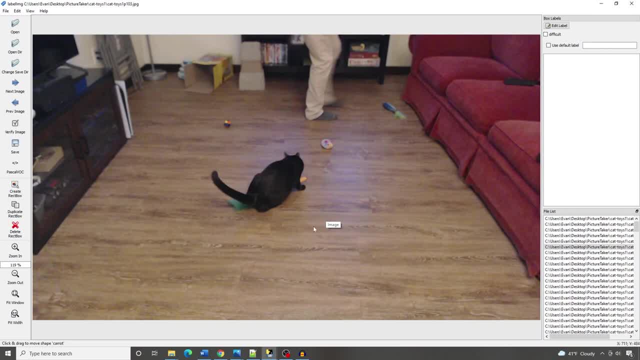 each end of the carrot past my carrot. If you're interested in learning how to do this, please visit the link in the description below cat's legs in this image. Should I label the carrot? Should I label the whole thing Or should? 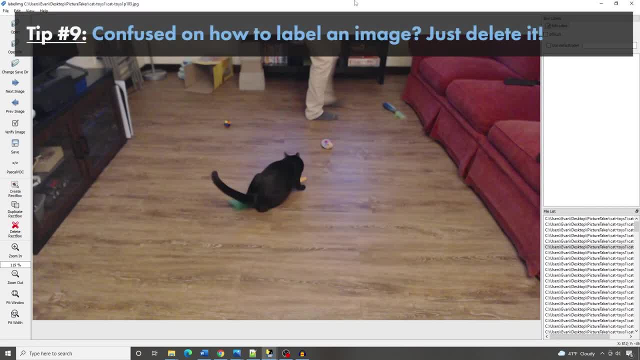 I label each end separately. My general rule is this: If I'm confused about how to label the image, then I just throw it out. The model learns best from clear, obvious examples. If you have confusing or contradictory labels, the training algorithm won't be able to minimize the model's loss.